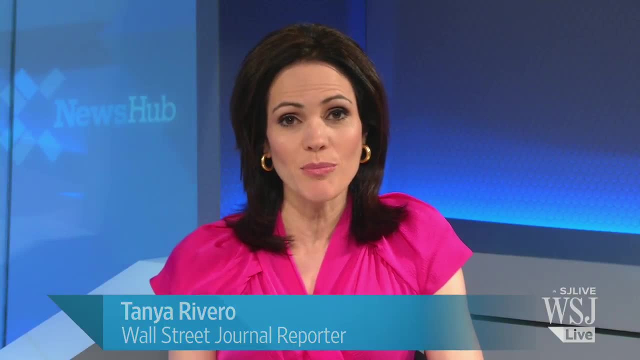 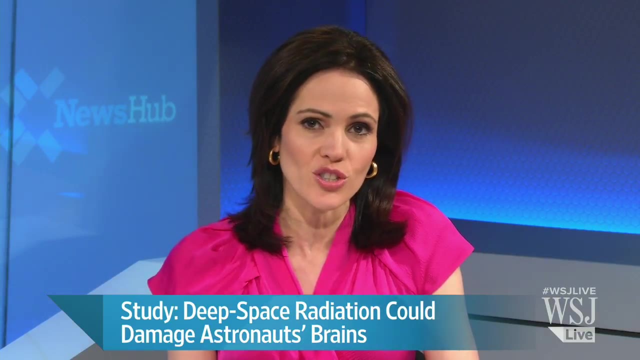 We may be living on the cutting edge of science, but a manned flight to Mars may be even riskier than previously thought. A NASA-funded study finds exposure to radiation during a journey from Earth to Mars could cause subtle brain damage in astronauts. WSJ Senior Science. 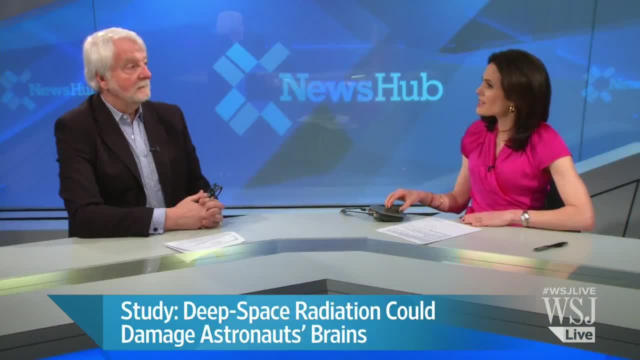 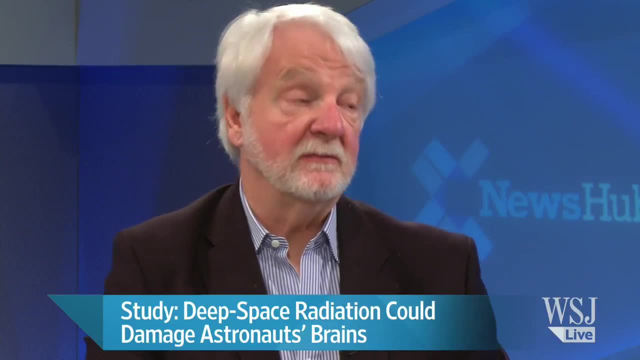 Correspondent, Lee Holtz, joins us now. Lee, thanks so much for being with us. Tell us about this study. What did it look at and how did it come to this conclusion? Well, space travel is inherently a risky business, but NASA and other space agencies that want to put people on other 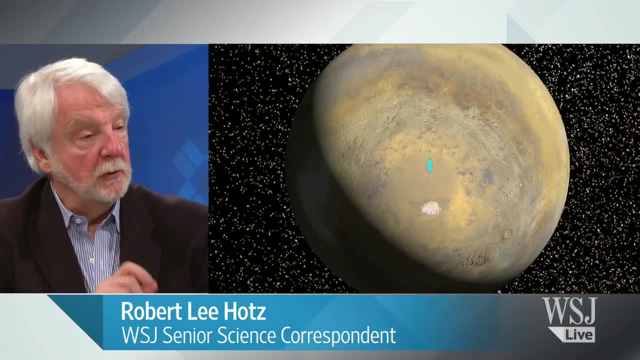 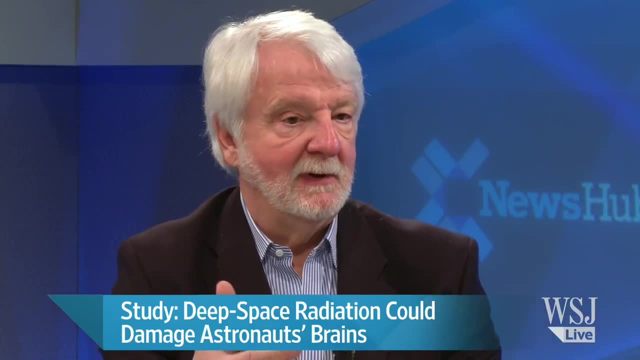 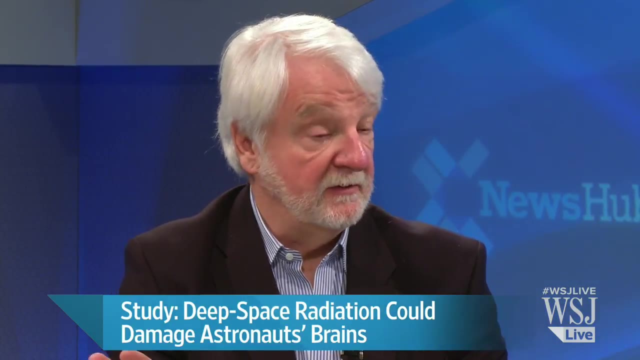 planets now have got something new to worry about: Long, prolonged exposure to the very low levels of radiation of cosmic rays. These are charged particles spewing from newborn black holes, from exploding stars far, far away. That floods the inkiness of space and the gaps between the planets And over the long periods that such a journey would run, space travel has been required to Mars, say a year, maybe three years. It could dumb you down. And the distance between Earth and Mars is what? about 140 million miles? A close approach? yes, It can get as far. 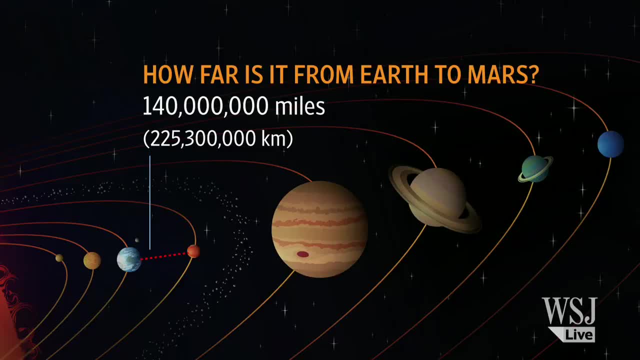 away as 300 million miles, But that means a journey, say, of a year or more, And slowly, gradually, over that period of time. researchers at the University of California at Irvine and University of Nevada, working with NASA funding, tested mice. 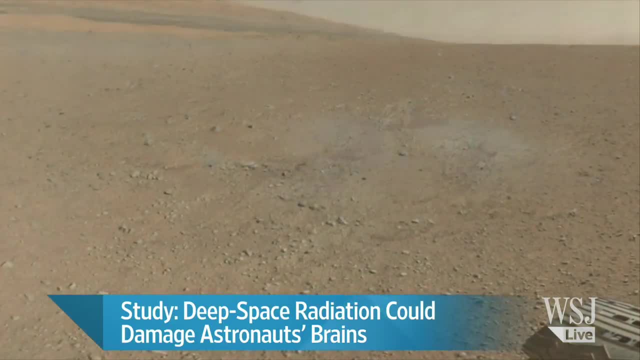 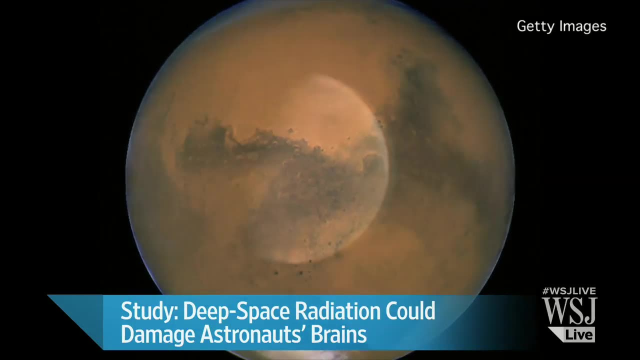 And radiation beams at Brookhaven National Laboratory out on Long Island, And what they found was that, after they exposed these mice to the kinds of charged particles you might encounter in deep space. Now we're not talking about where the space station is or where the space shuttle. 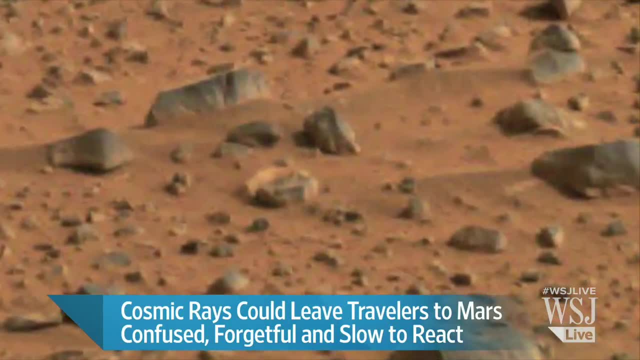 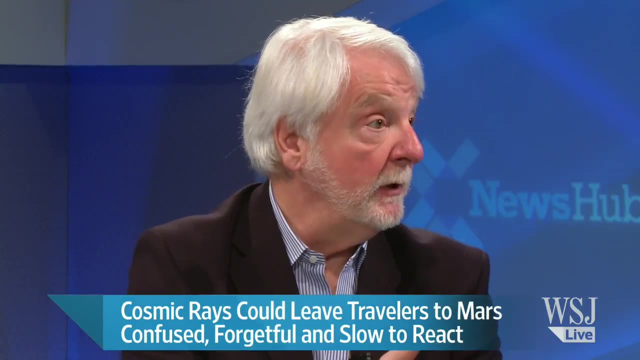 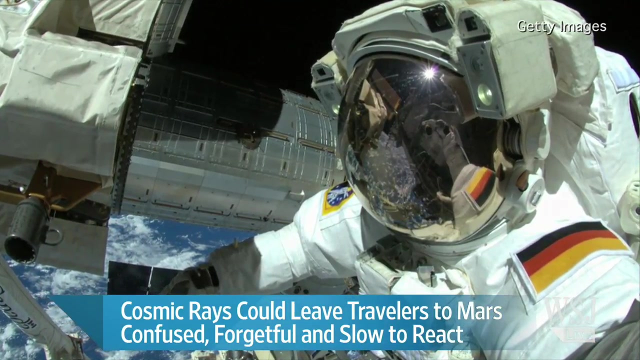 pilots used to fly. That could have serious effects on your brain cells in your hippocampus, in your prefrontal cortex. These are all areas associated with memory, with decision-making, And literally the particle, The particles appear to sort of break off pieces of the synapses And it has the consequences on 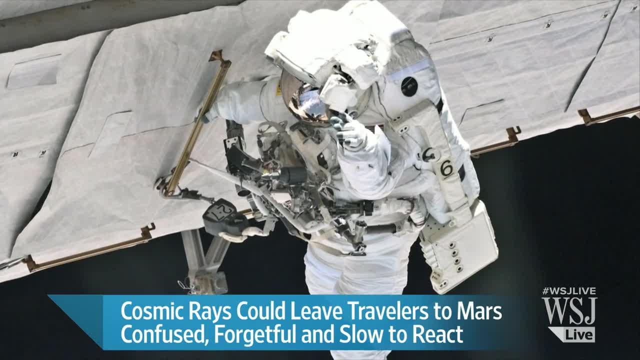 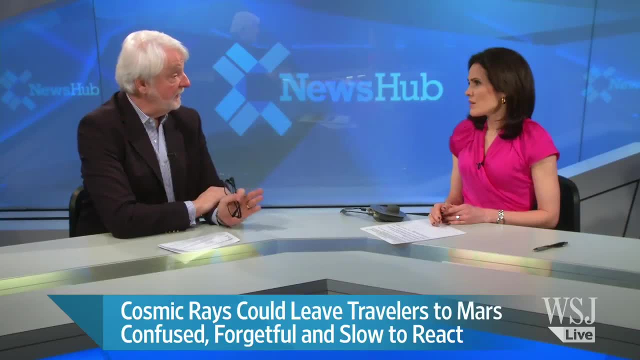 behavior. You get slow, You get easily confused, You have trouble remembering. I mean, we send some of our smartest people into the astronaut corps and into space And this is going to shave points. they say perhaps off their IQs, This could be dangerous in a spaceflight emergency.